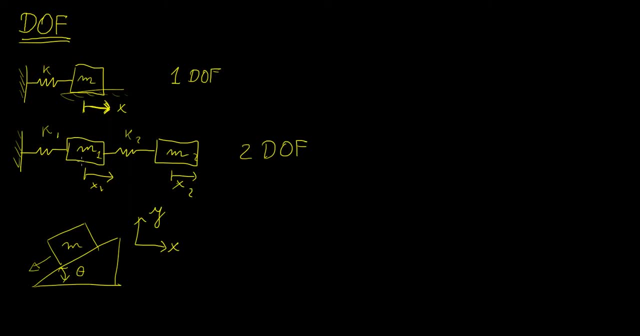 in the end, because we're taking into account just individual motions happening. then we say that this system has two degrees of freedom. Now, in the same way, we could actually assume that we have the following case: So imagine that you have a flat surface and then you have something like a disc on top of 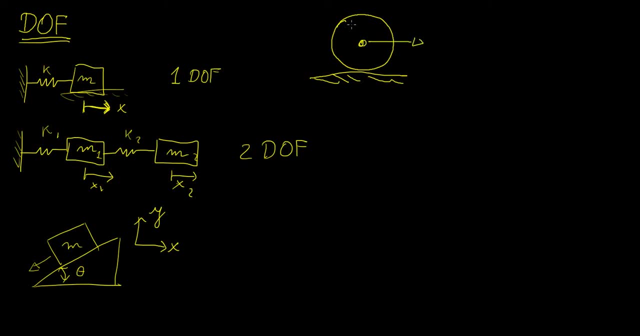 it. and this disc is moving to the right, and it is also rotating, so there's no slipping happening. Now, how many degrees of freedom do you think the system has? Well, there are two, essentially two ways in which this disc can move. It can 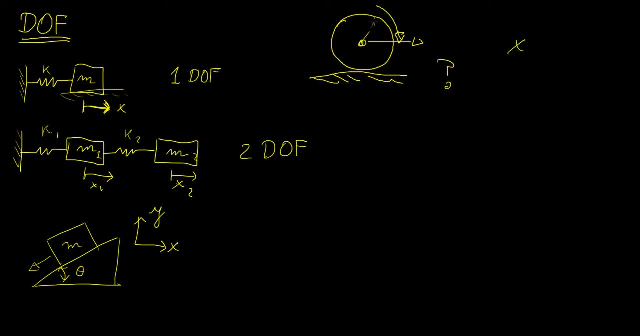 either move along the x-direction or it can actually move in terms of angular displacement. So there is some angular displacement happening and in the end we have two types of motions. We have translation and then we have rotation, but there's only one of each of those. So in the end we say that this system here 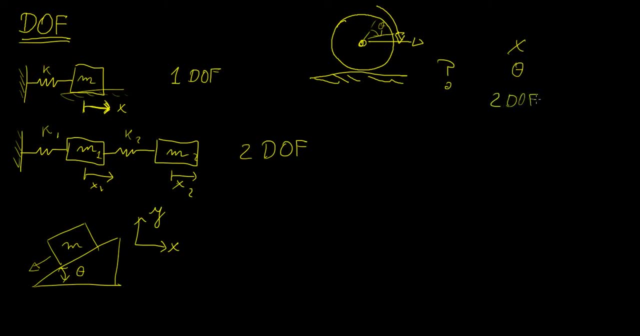 has two degrees of freedom, because it is essentially free to move in two different ways and it actually moves as a combination of both. Now, degrees of freedom are important because you need to identify exactly what are the equations of motion that you're going to get. You can get an idea of the kind of 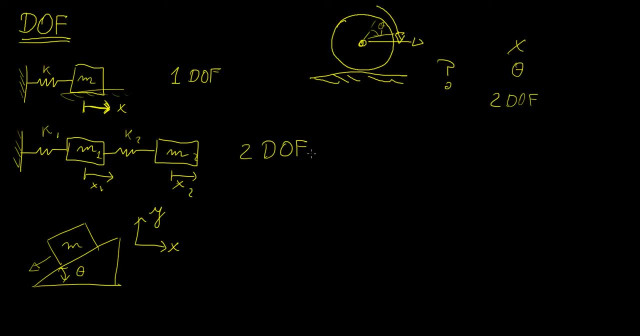 equations of motion simply by looking at the number of degrees of freedom. So you should have an equation of motion for each degree of freedom. That's the general idea behind it. Now, there are some cases in which things might not be as obvious as others, so I could give you this example here, where you have an 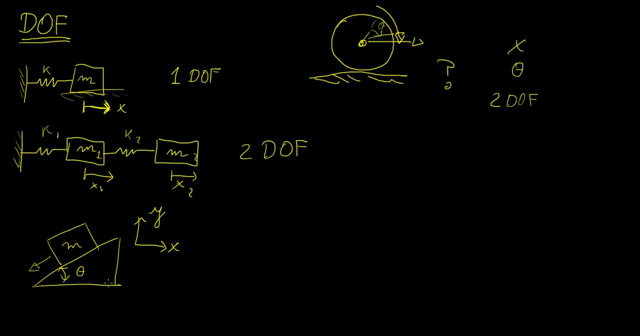 inclined plane and then just a mass resting on top of it. Now, if the mass starts moving along the surface, here you might think. well, there are two directions in which this is moving. This is not only being displaced along the x-direction. 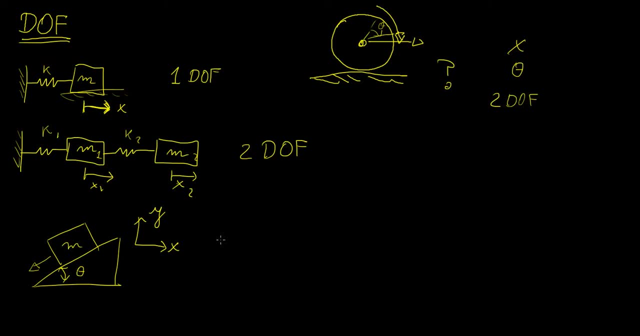 but also being displaced along the y-direction. So you might be inclined to think that this system here has only two degrees of freedom, but the thing about degrees of freedom is that we can always find a way to simplify things. So in this case, in this reference frame, yes, it looks like this system has two degrees. 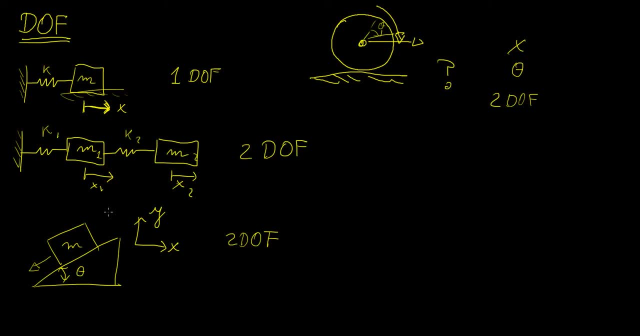 of freedom. but if we shift the coordinate system and perhaps do something like this- Let's say we rotate the coordinates and now we create a new set, x prime and y prime- Then look at what happens in that case. In that new reference frame, this mass is only moving along the direction. 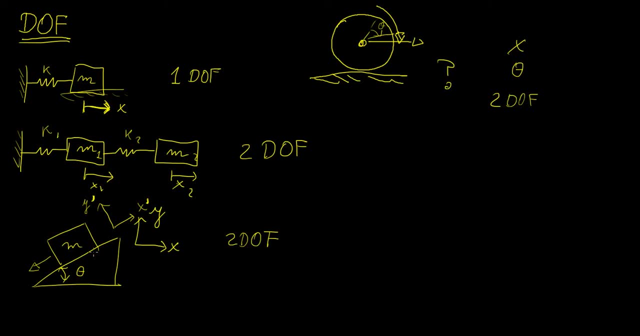 parallel to the surface, It is not really moving perpendicular to it. So you might think well which one is the correct one to choose in this case, And it turns out that you can choose either. but in general, what's simplifies your analysis is the minimum amount of degrees of freedom in the system. So if you 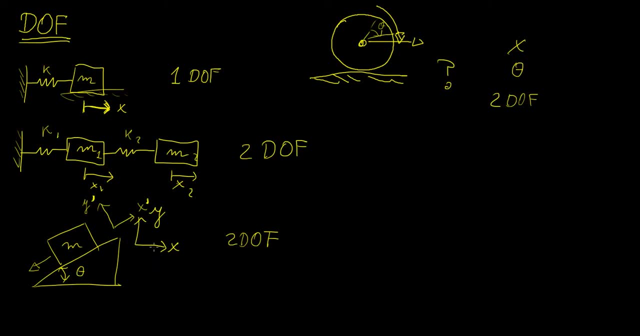 can go from two degrees of freedom to one degree of freedom, then that means that you can pretty much simplify the calculation, so you can simplify the whole process of deriving equations using Lagrangian mechanics. So in general we tend to do this kind of thing. If we find a way to 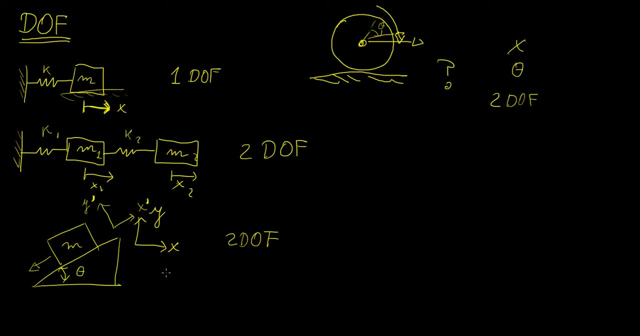 reduce the number of degrees of freedom in the system, perhaps by some coordinate transformation, then we do so first, and then we apply the analysis and you find out that it actually is quite a simplification. So this kind of thing is really useful to do sometimes, and we'll do some. 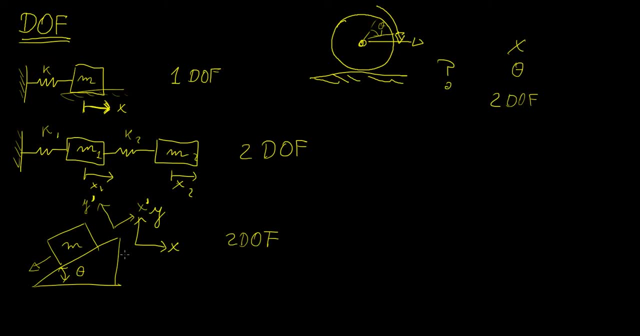 examples with this later on, just to show you exactly what this whole process looks like In general. it doesn't matter whether you solve it using this reference frame or that reference frame, because Lagrangian mechanics actually works in any reference frame. It is invariant. 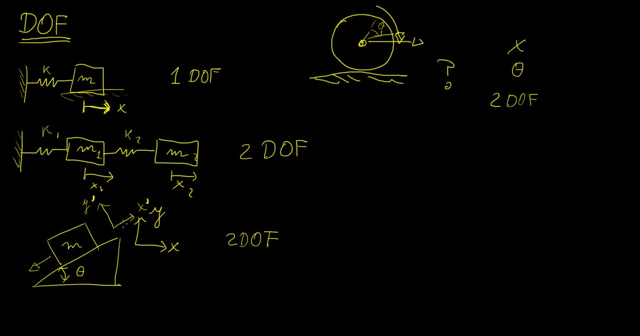 of coordinate systems. But you will find out that by reducing the number of degrees of freedom you actually simplify the problem and make it easier for you to derive the equations of motion, because in the end you know there is a relation between this coordinate system and that, So you can just 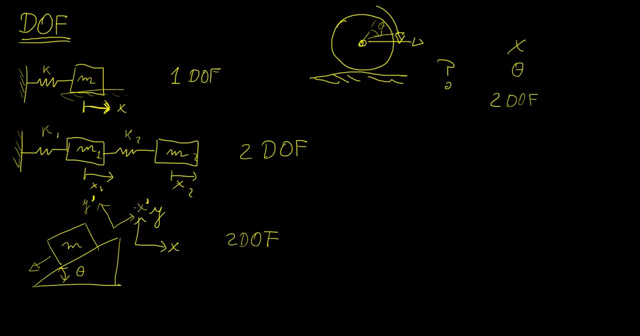 relate the coordinates of those equations of motion back to the original ones simply by performing a substitution. So we'll talk about that as well. Now let me give you another example. So we're going to have something like a simple pendulum, And this is exactly what we analyzed in the previous video. We had a mass 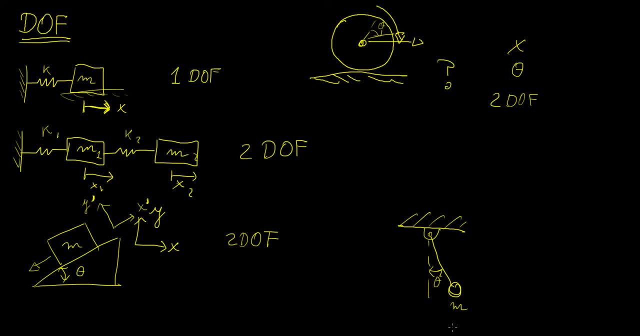 hanging from a rod and then the rod. it was just oscillating back and forth. Now you might think: well, if you look at the problem from the reference frame of the bulb, you might be inclined to say that it is actually moving in two directions. So in that case you might say: well, it is moving in. 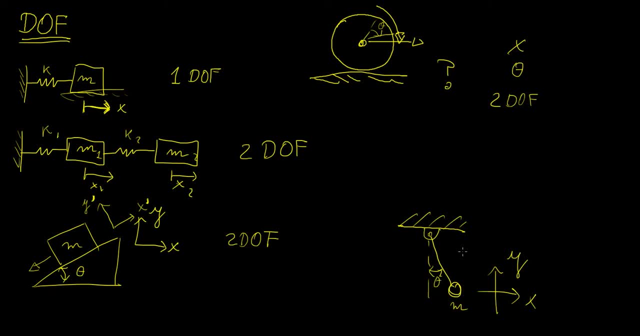 it has two degrees of freedom, right. So you might say: well, it has two degrees of freedom, right. It's moving along the x direction and along the y direction as well. But there is also another possibility: If you look at the whole system as just a single arm that is just swinging back and 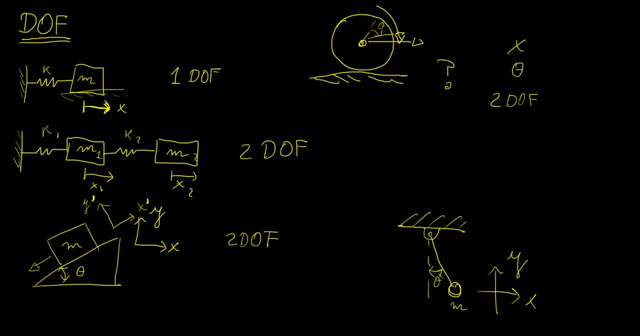 forth about a fixed pivot point, then what you notice is that you can express the total motion of that system in terms of that angular displacement. So, instead of taking into account two degrees of freedom, you can take into account the angular displacement, rotation motion, And this is essentially being able to describe the angular displacement of the節目 of the tudo gebeah. 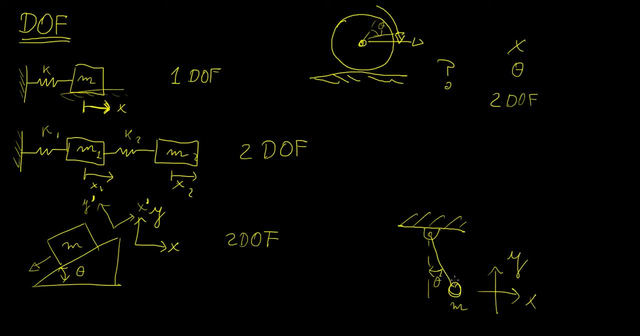 Instead of taking into account the angular displacement of the pendulum, and this is essentially going to give you what you need in order to analyze the problem and make it a lot simpler. so, in general, we prefer to just go with the minimum amount of degrees of freedom, so look for the minimum number. look how you. 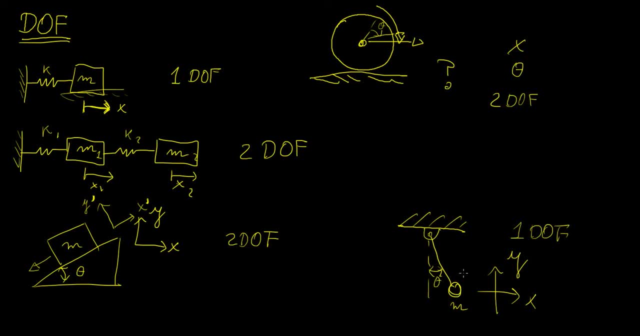 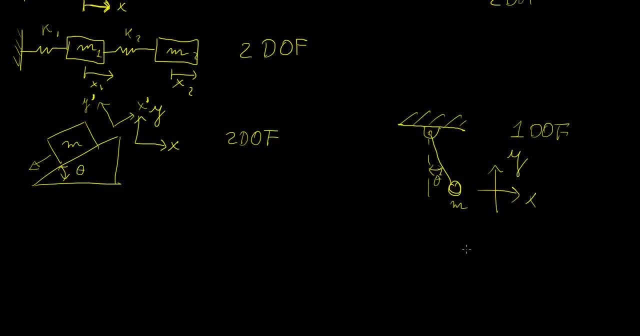 how you can simplify the problem before even starting to solve, and then you'll see that the process is a lot quicker and a lot easier. so, in the same manner, I could give you the following: I could give you a double pendulum system, and this is something that we will also study in this playlist. so you're gonna 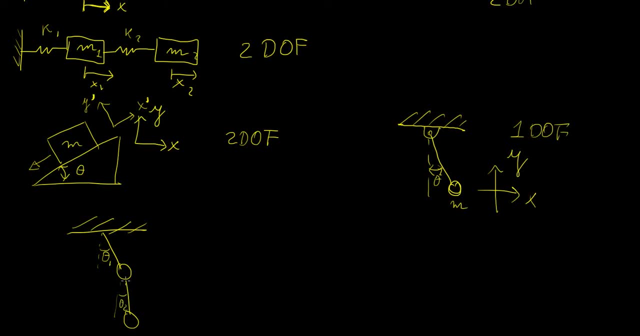 have two angles, something like this: you have two masses here. now you will think, well, maybe this has four degrees of freedom. this one can move in two ways, if we can move in two ways. but we know that we can completely characterize the motion of both simply by using their angular displacement, because the 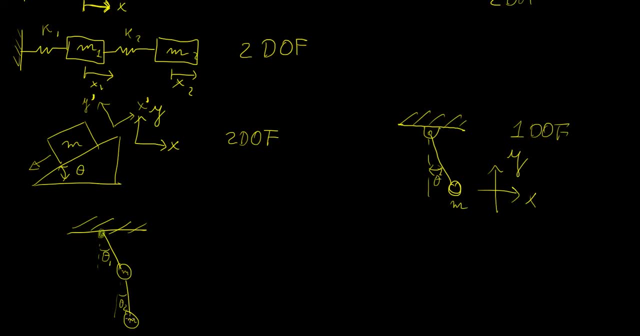 rotation is the same as the rotation of the pendulum, so we can move in two ways. this one is rotating about fixed points, this one is rotating about a fixed point. this one is rotating about this one's frames of reference, but as far as it is concerned, it is fixed with respect to this one. so in this case we still have.